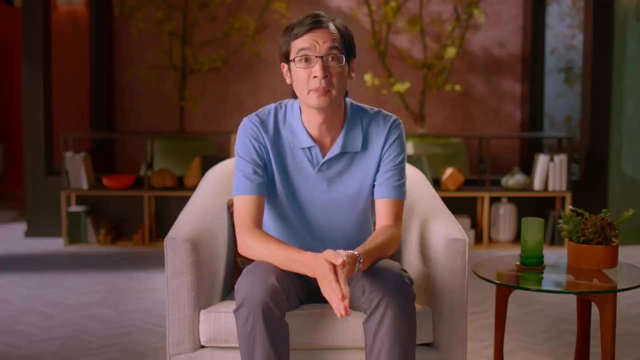 to the way we learn math. But I think we all have an innate ability for mathematics. 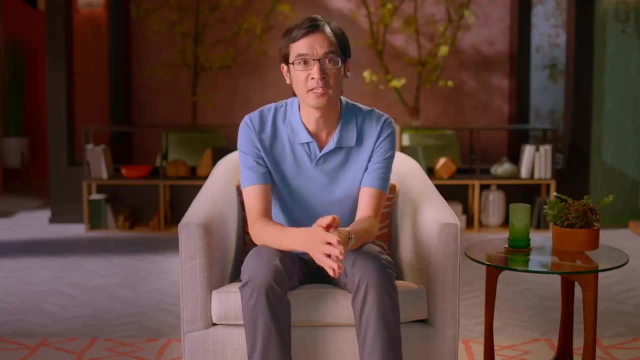 Knowing how to think mathematically can be a tool that you can use to solve problems in a systematic way. I like to think that this class is for anyone really. In fact, maybe this class is even more suitable for people who have not had formal mathematical training. 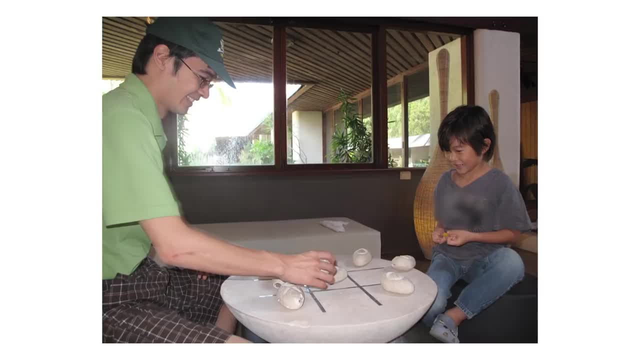 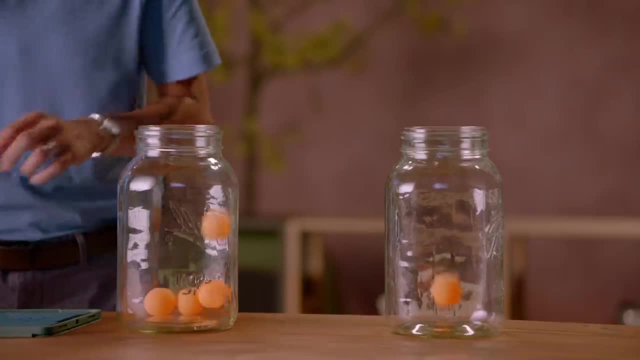 I'm not going to give you homework. The way I approached problems in mathematics was to try to turn it into a game. A large part of this class will be about talking about problem solving. We abstract them, we break them up into pieces, we make analogies, we try to find connections between them, and then we try to solve them in a systematic way. It's a lot of fun. 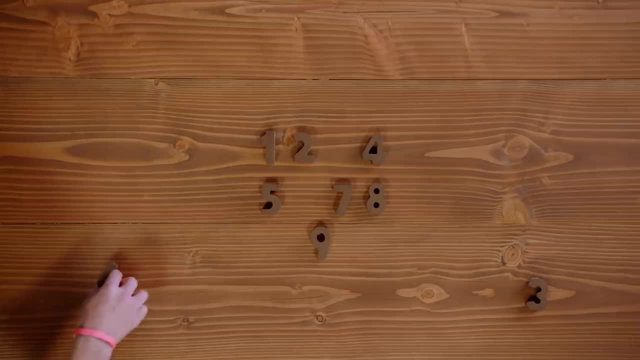 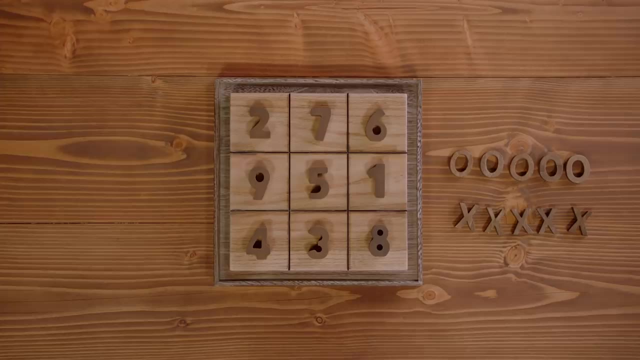 The first player who can collect three numbers that add up to 15 wins the game. Playing this game is quite challenging if you don't know the trick. You can transform this to a much more familiar game. Tic-tac-toe. People often anthropomorphize mathematical objects. They 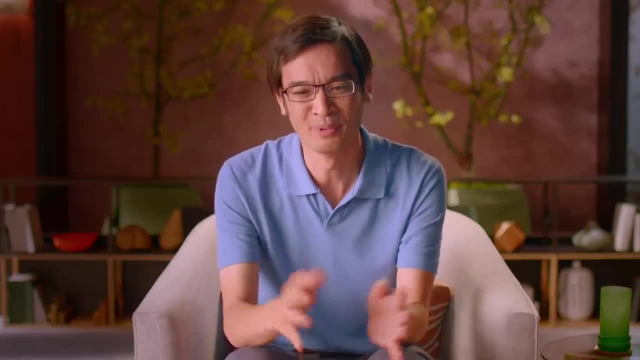 call this guy the enemy, this guy is your friend. Some people call them slightly more obscene names. 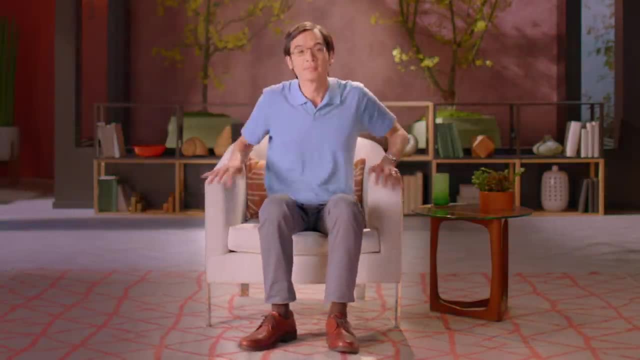 In this class, you'll appreciate a little bit more what mathematics is, how we solve problems, and how someone with these strategies can be of use to you in your daily life. 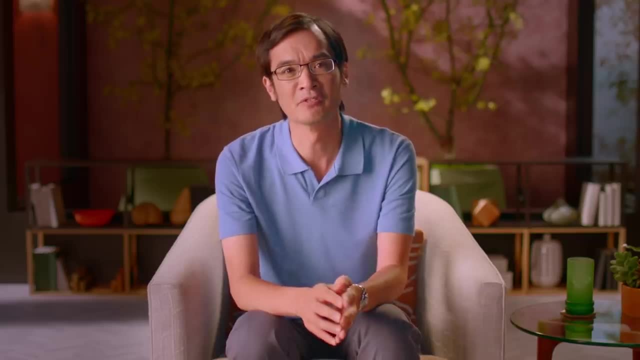 The ideal problem to work on is one which is just barely outside of your reach. 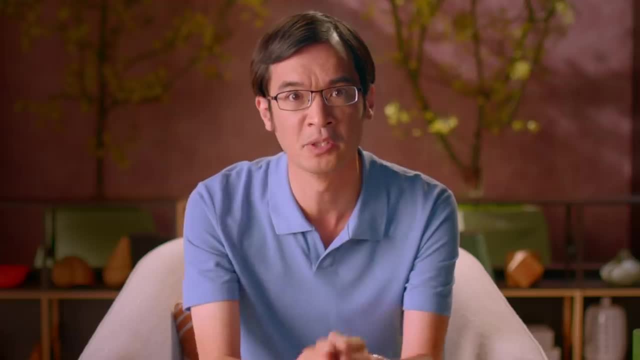 It's not so much whether you succeed or fail at a question, but it's whether you can learn something from it. My name is Terence Tao, and this is Masterclass. 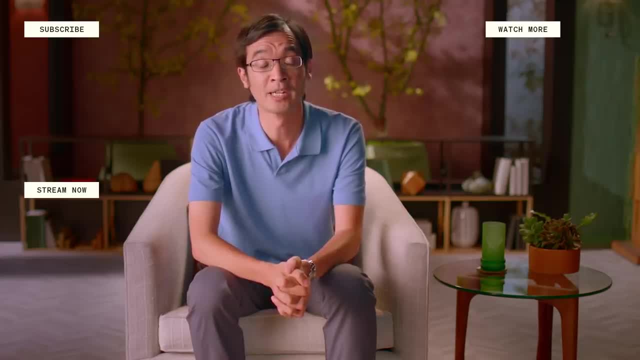 I'll see you next time. 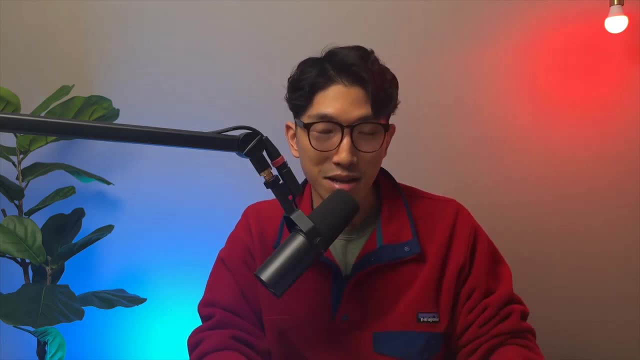 Whenever you're taking the SAT or any kind of exams in class, the exam's looking a little rough and you're about to be done with the first question and there's like 10 more questions to go. All of a sudden, out of nowhere, you suddenly hear a student across the classroom flip to the second. 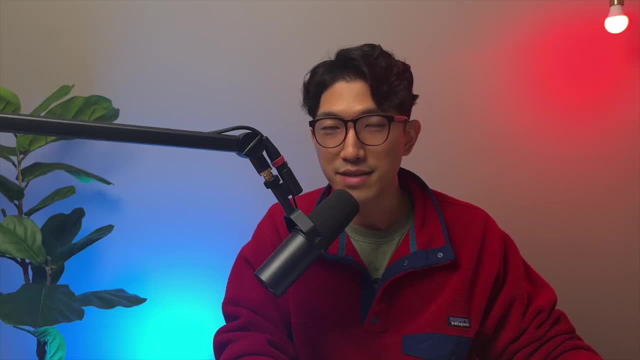 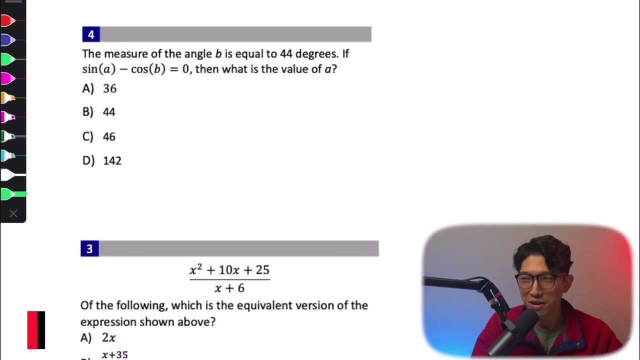 page. Then everybody goes: what the f**k? And in today's video I'm going to show you how to become that student. It's always fascinating and kind of frustrating on how we all learn the same thing and we are all in the same class And it's entirely possible that that student is smarter than you.